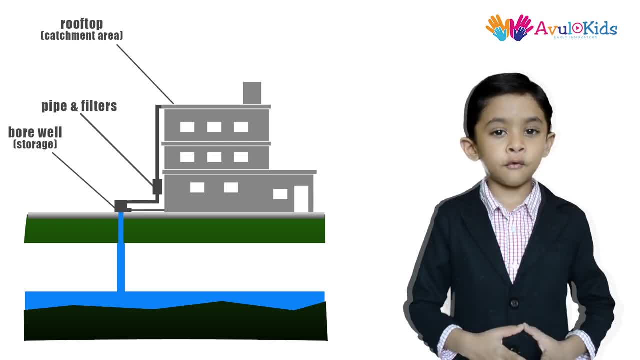 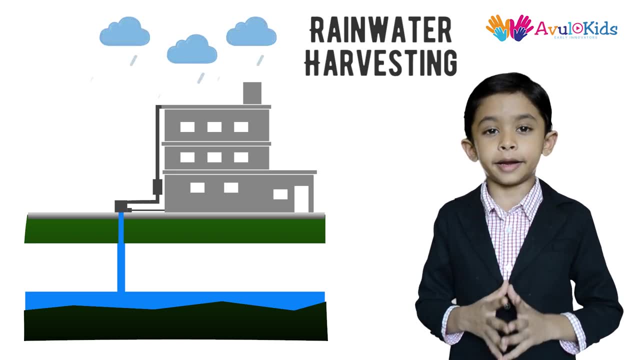 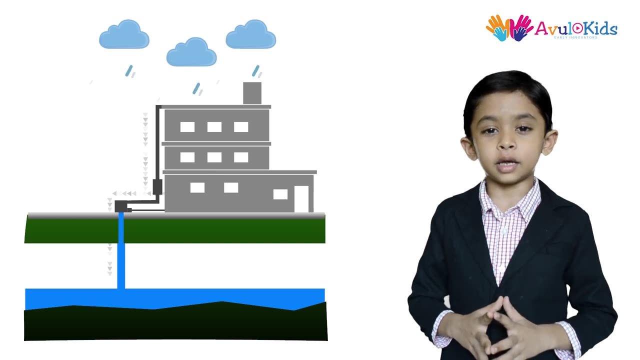 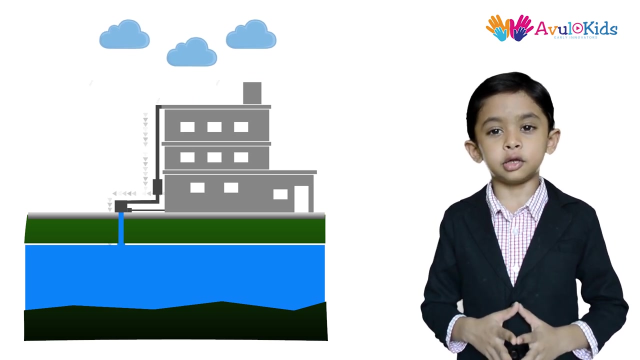 And use it through wells and bores for rest of the season. This process of saving the rainwater in ground is called rainwater harvesting. All the rooted water can be collected and sent it in the pits, wells and bores. This recharges the groundwater and groundwater can be used throughout the year. 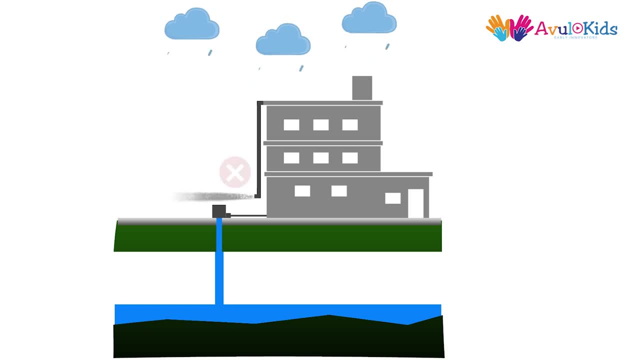 To save the rainwater, it is necessary to store water in the pits and then store the region where it gets wet. Sea water must be stored under the wet, clear field, under dry soil and under clean water. The rainwater can be stored in a layer or container, be it water pump, water pump, paperaran water pump, as well as other products to help preserve the rainwater. 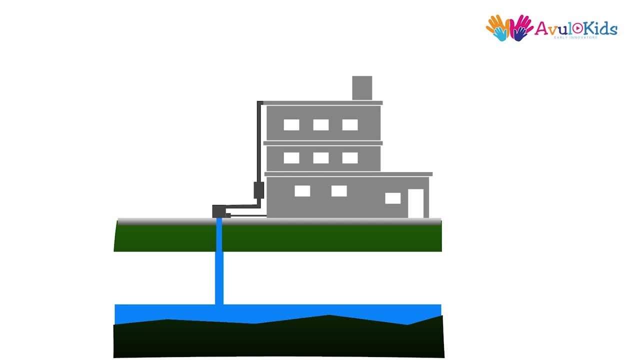 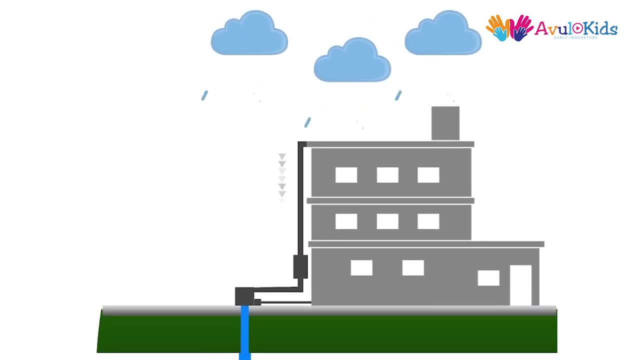 This is all because of the lack of water. In third part, let us see how we get the fresh water. In third part, let us see how we get the fresh water. In third part, let us see how we get the fresh water. 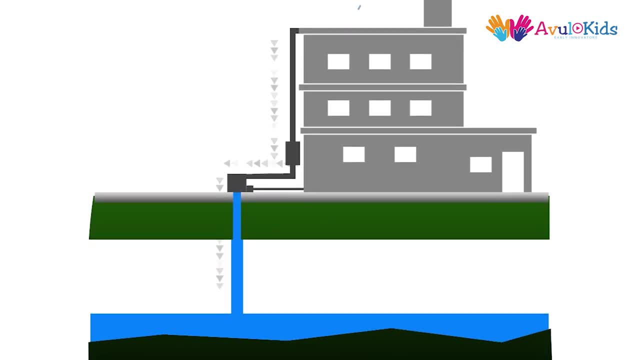 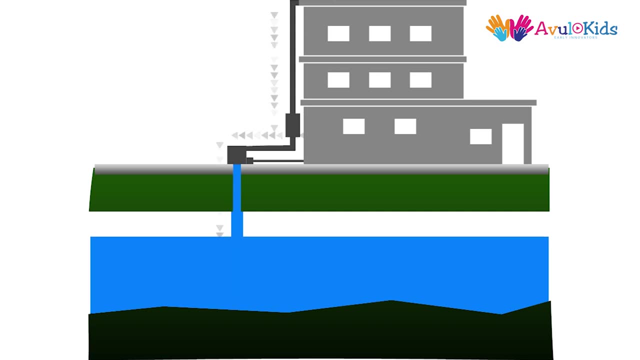 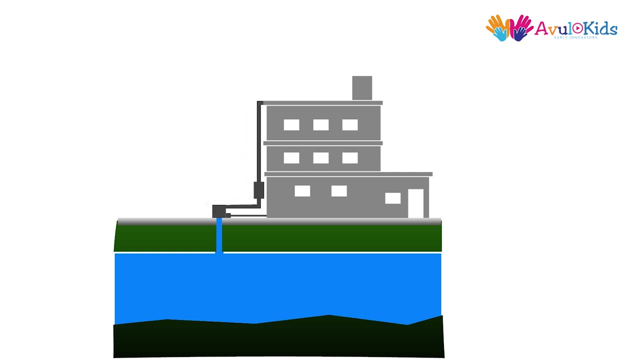 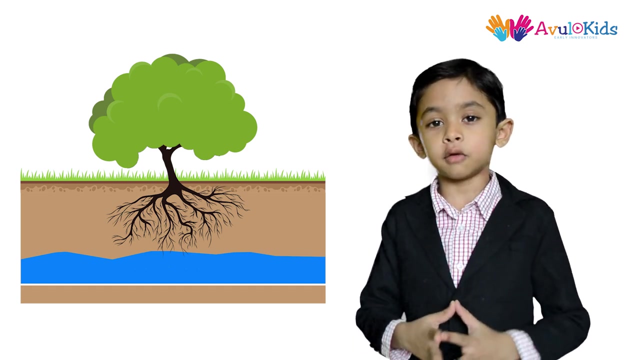 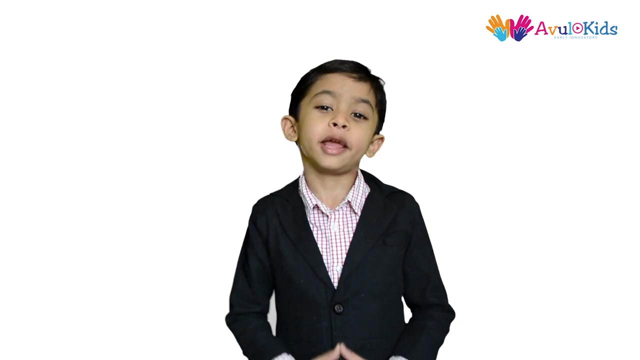 Do you know trees also use ground water to grow. is it not the simple way of saving the rainwater and use it for rest of the year? Friends, if we don't save water today, most of us will not have enough fresh water when. 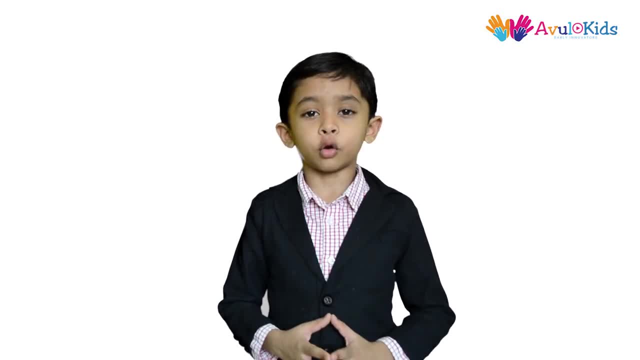 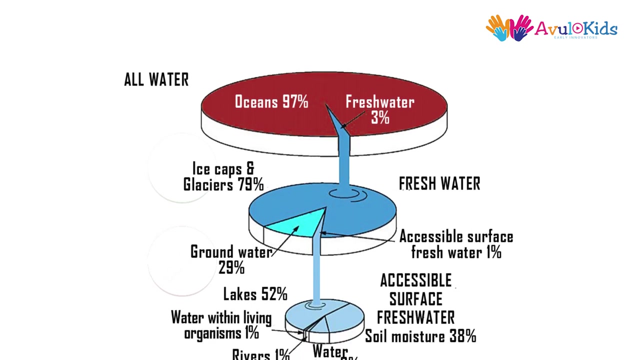 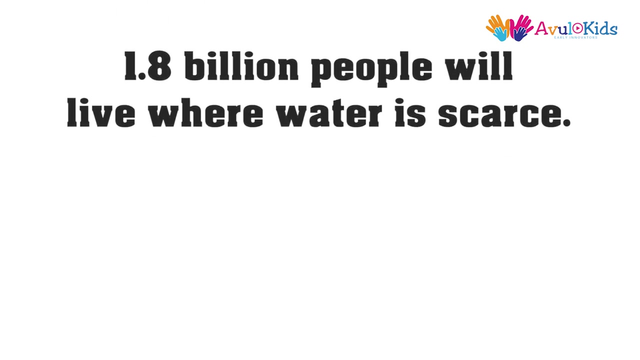 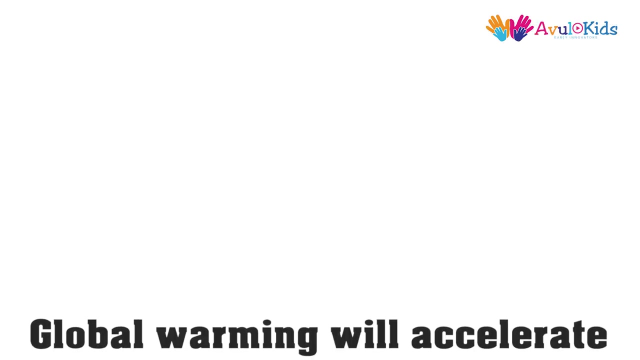 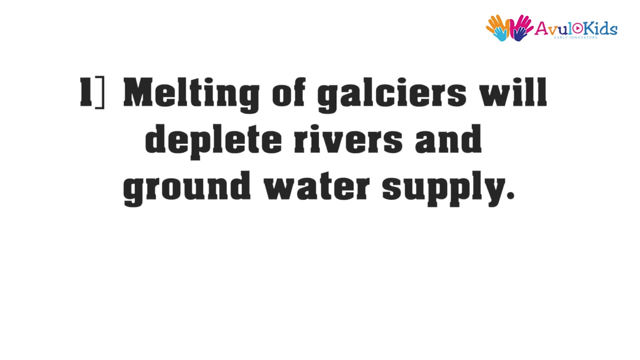 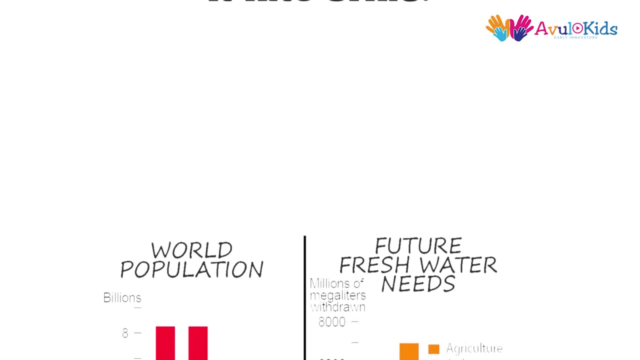 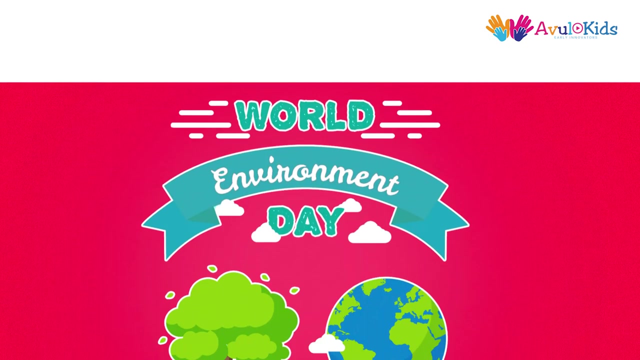 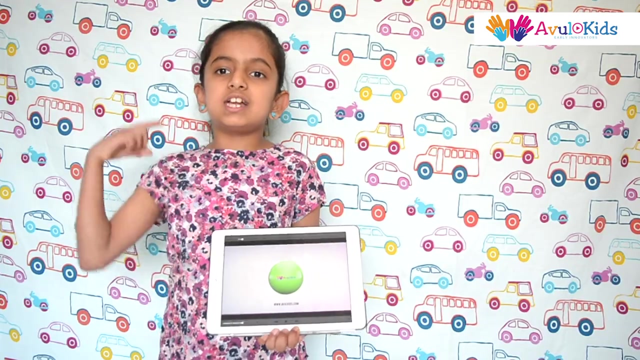 we grow up. So let us start saving the water for today while making rainwater harvesting. Hope my video was of service to you. Thank you for watching my video. Bye, See you next time. Please like and share our video and subscribe to our channel.